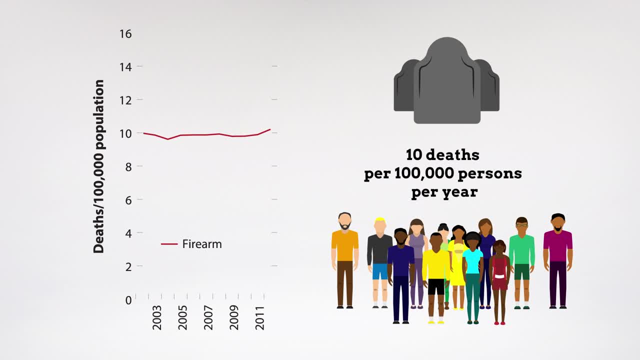 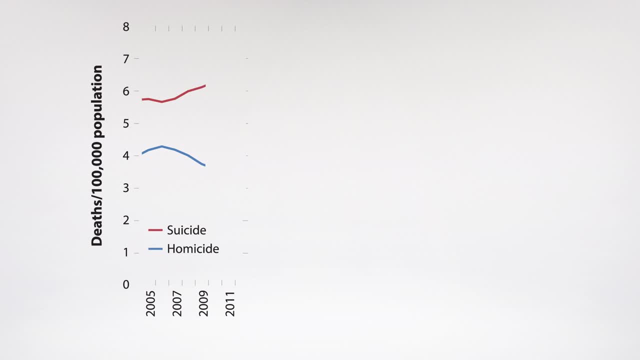 this stability masks a notable divergence: Firearm homicides have decreased since 2006, while suicides have risen by the same amount. Suicide has been the most common form of fatal gun violence over the past 30 years and, in 2012, accounted for 64% of fatal firearm violence. 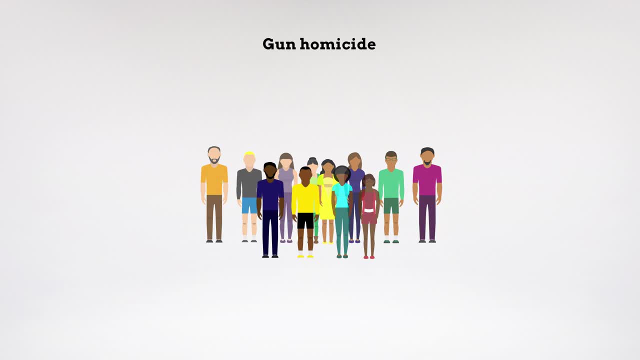 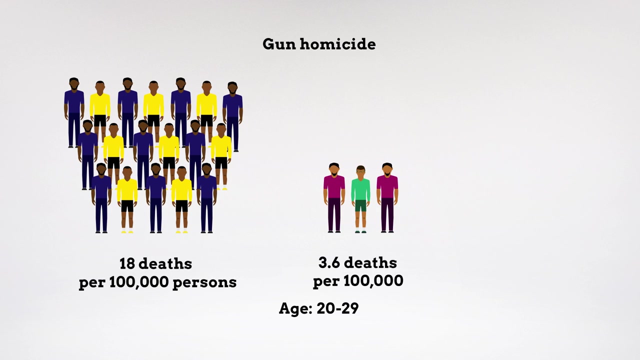 Gun homicide is concentrated to a remarkable degree among black males, especially young black men. In 2012,, the gun homicide rate for black males aged 20 and older was almost 18 deaths per 100,000 persons, which is five times higher than that for Hispanic males and 20 times higher than that for white males. 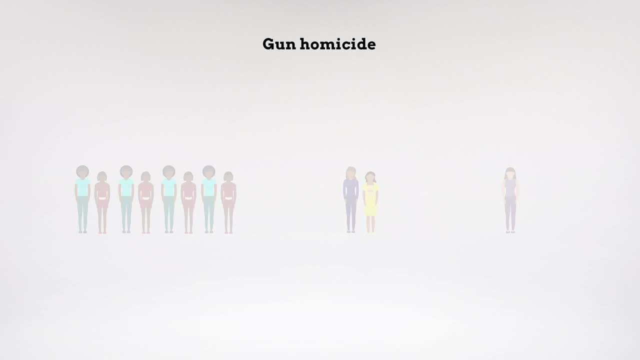 The pattern for firearm homicide among females is similar to that for males, but the rates are lower by a factor of 10.. Black females aged 20 to 24 had the highest mortality rate in 2012,, with approximately 7.5 deaths per 100,000 persons. 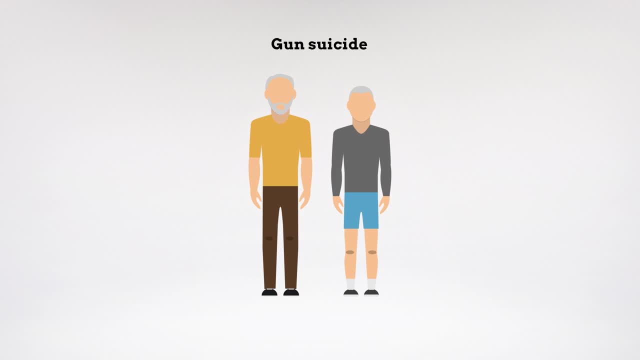 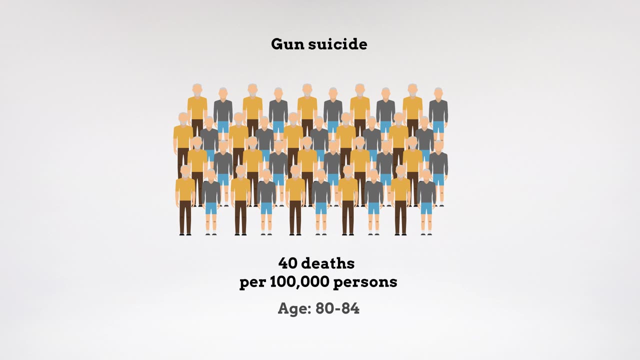 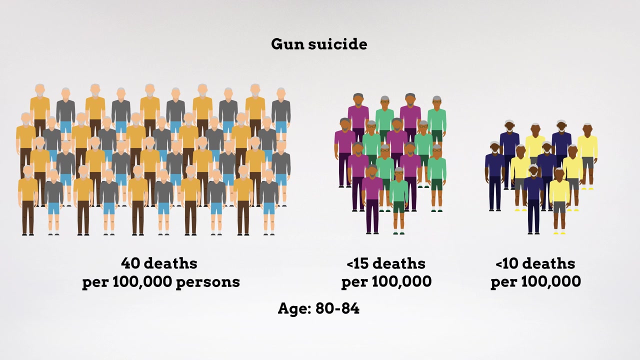 The risk of gun suicide, on the other hand, is highest among white males. In 2012,, suicide rates for white males peaked at 40 deaths per 100,000 persons among 80 to 84-year-olds, while the rate for Hispanic men was below 15, and that for black men was below 10 per 100,000 persons. 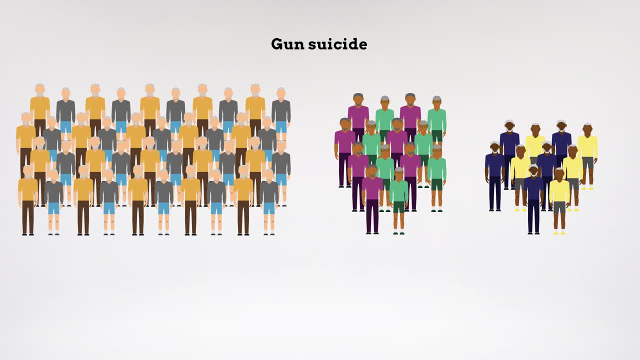 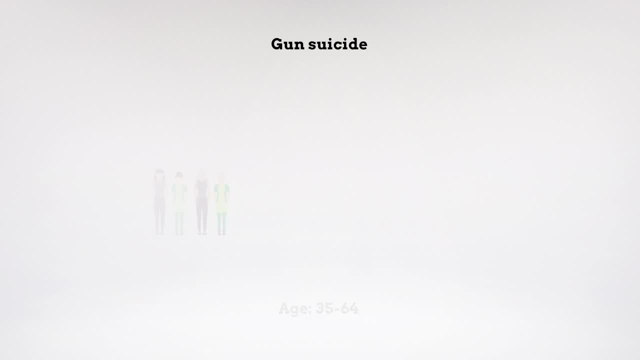 Between 1999 and 2012,, the death rate due to firearms increased among white males aged 35 to 64 by almost 36%. White females are similarly more prone to firearm suicide than black or Hispanic females, although the number of cases is lower than male cases by a factor of 10.. 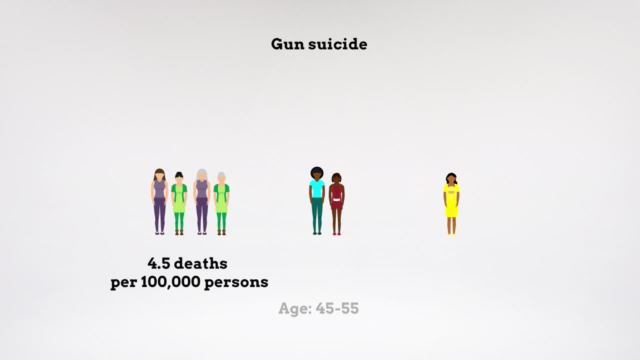 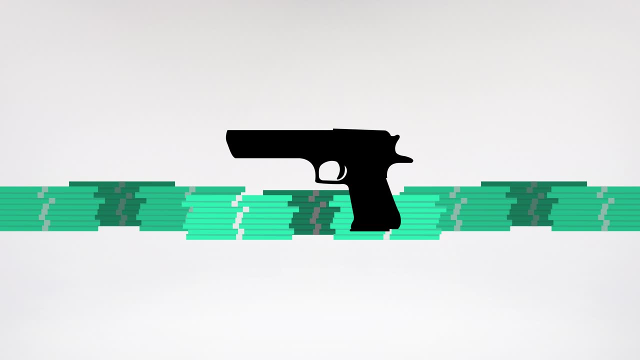 It peaks at 4.5 per 100,000 persons among white women aged 45 to 55.. The societal costs of firearm suicides and homicides are enormous. For 2010,, the estimated cost was $164.6 billion, approximately 1.1% of the US gross domestic product for that year. 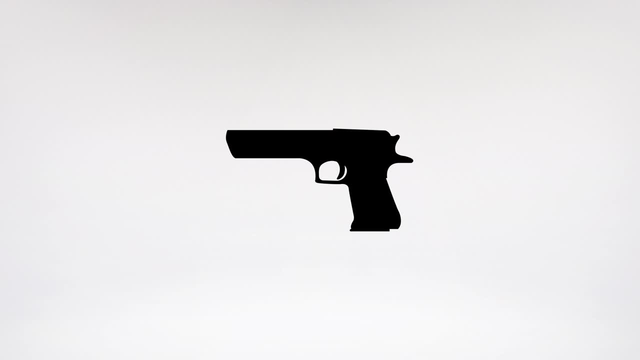 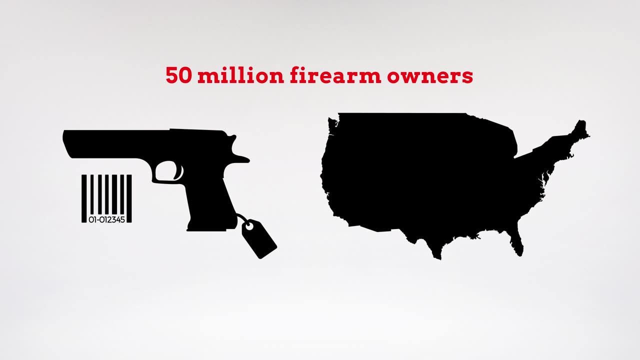 While there are many factors associated with the risk of death from firearm violence, the most widespread appears to be gun ownership. The US is home to more than 50 million firearm owners. Approximately 35% of men and 11% of women report owning firearms.